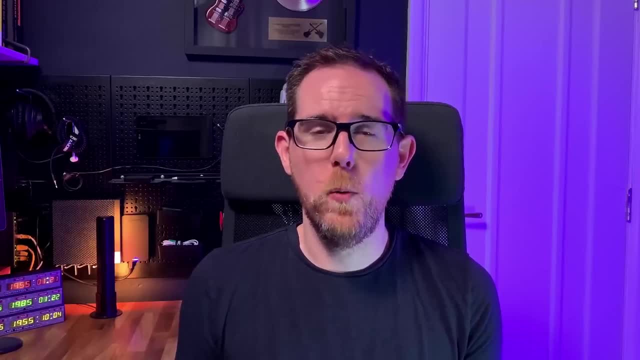 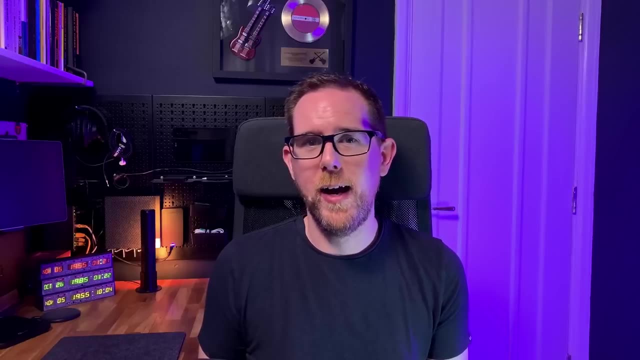 analogy will help. So let's say it's my birthday tomorrow and my wife is going to bake me a birthday cake. To do this, you might follow a recipe, and this is going to give a step-by-step instructions on how to bake that cake. The recipe, in this case, is an algorithm it's giving you. 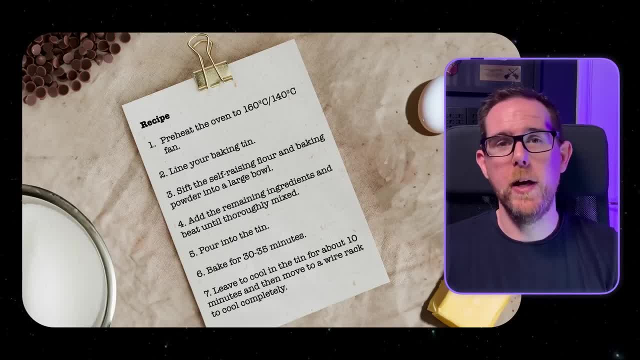 step-by-step instructions on how to bake a cake or how to cook cake. It's a run on different on how to bake a cake that you can repeat over and over again to produce the same thing. Sure, you might switch out some of the ingredients to produce different cakes. 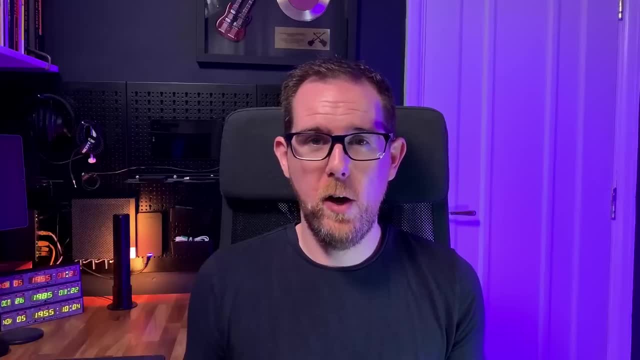 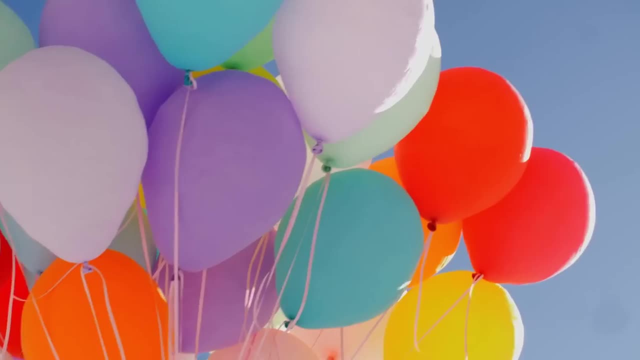 but these are really just different input variables. As it's my hypothetical birthday, I also want to have a birthday party. Now, if you think about a birthday party in your head, you're probably thinking about balloons and banners and maybe someone with a cake with candles on it coming out. At least, that's what you are. 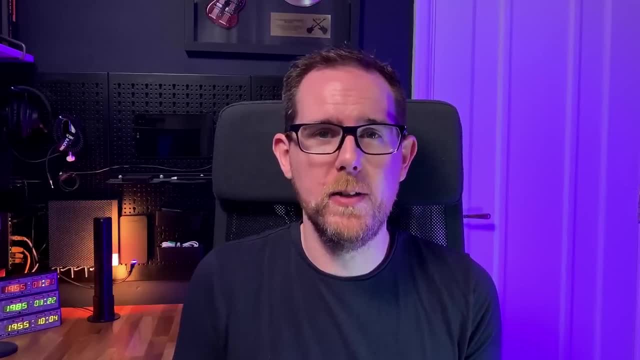 thinking about now. But everybody's idea of a birthday party is going to be different. There's no set steps to follow, There's no recipe like you have with a cake. Essentially, a birthday party is going to be different for every person. 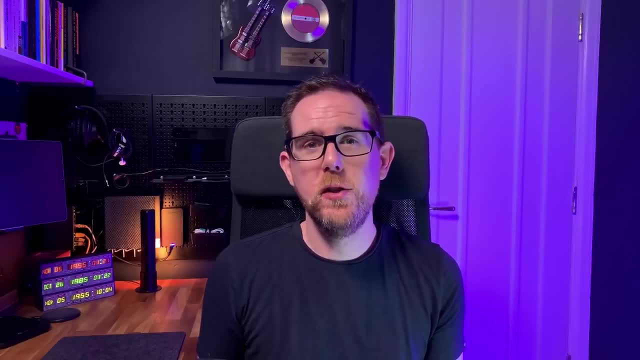 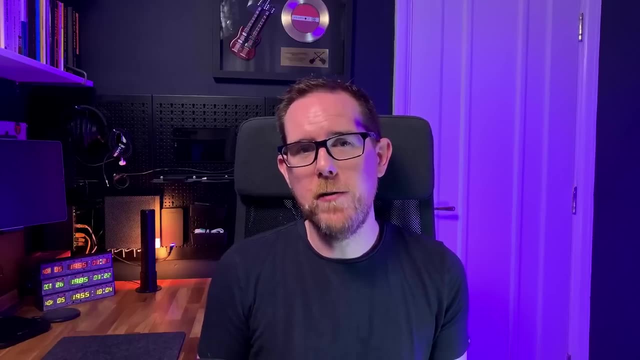 like the problems that we face in software engineering, But let's imagine that you have this amazing superpower that lets you see what everyone else is thinking. If everyone was thinking about a birthday party, even though they're very different, you would still recognise it as a birthday party. 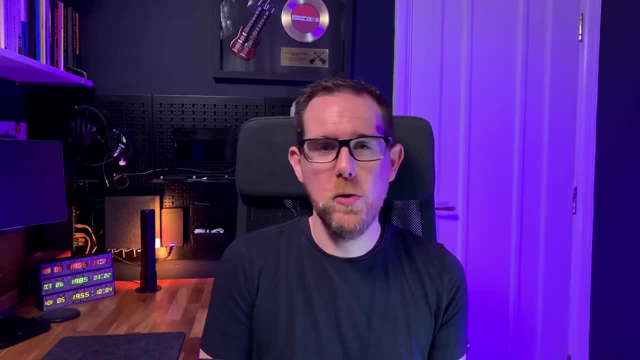 The birthday party in this case is a design pattern. It's the concept of a birthday party that can be reused, even if everything else is slightly different. Hopefully, you've learned a bit about the concept of a birthday party. Hopefully, you've learned a bit about the concept of a birthday party. 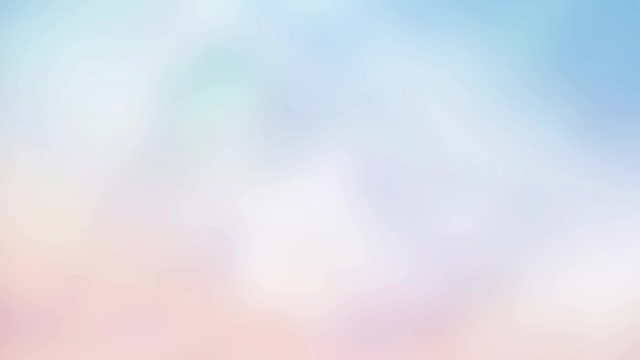 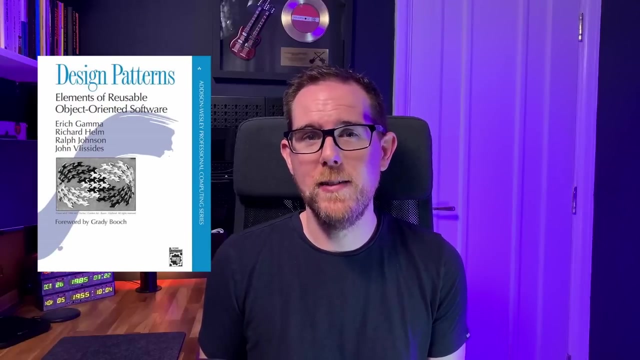 Hopefully you've learned a bit about the concept of a birthday party. Hopefully that analogy makes sense, But if it doesn't, let's have a look at what the design patterns actually are. In 1994, four authors wrote down 23 design patterns in the book Design Patterns. 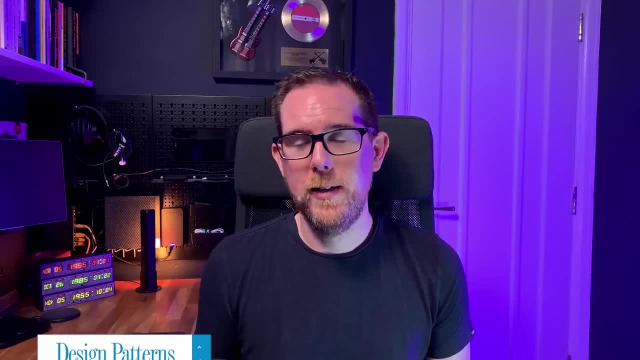 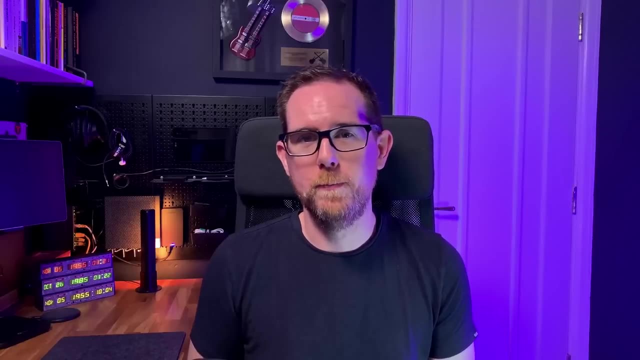 Elements of Reusable Object-Oriented Software. Now, obviously that's a bit of a mouthful. It's not something you can talk about at a party, for example, So most people call it the Gang of Four book. If you've been programming for a little while already, chances are you've probably already 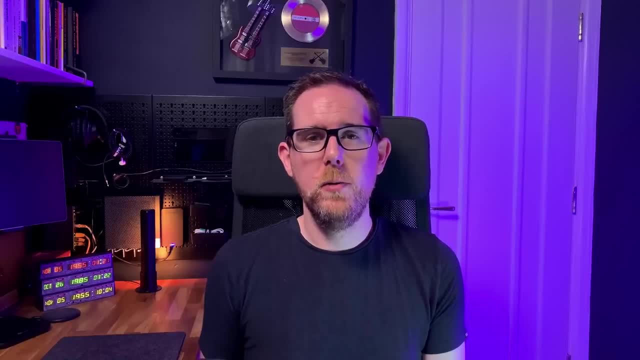 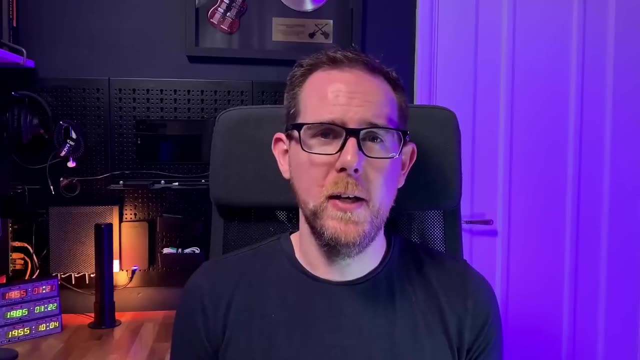 used some of the design patterns even without realising it. Most of them are just common sense, I know. when I first started looking at them I recognised them immediately for patterns I use in my own code, even if I gave them a slightly different name. So we have 23 design patterns. 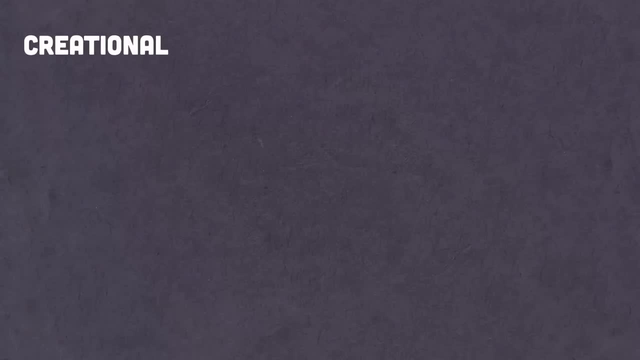 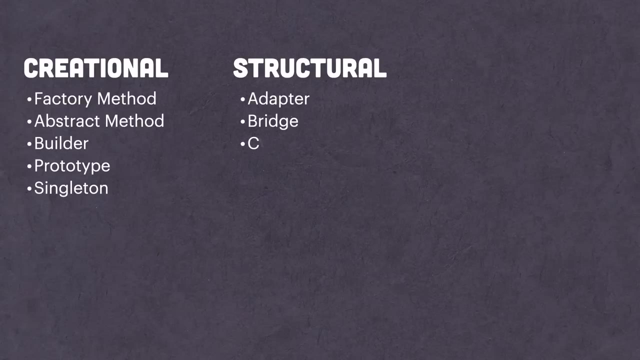 and these are split into three main groups. We have the creational design patterns, so these relate to creating objects in your code. We have the structural design patterns, so how we actually structure those objects, especially when they get quite large. And finally we have the behavioural. 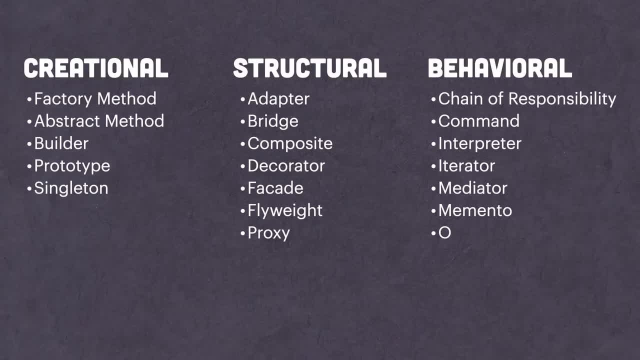 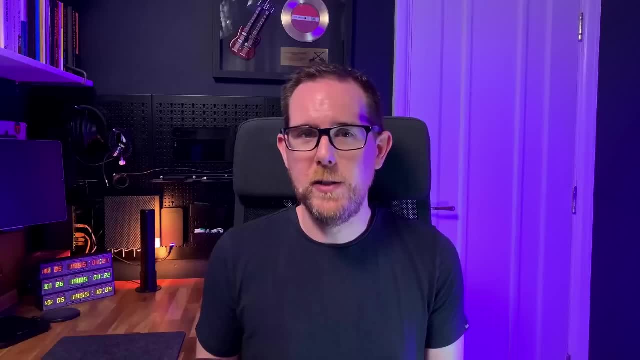 design patterns that covers the interaction between those objects and their responsibilities. Now you might be looking at this list and thinking, wow, I'm never going to remember any of those, But no one's really expecting you to know all 23 design patterns. But it's worth looking through them all. 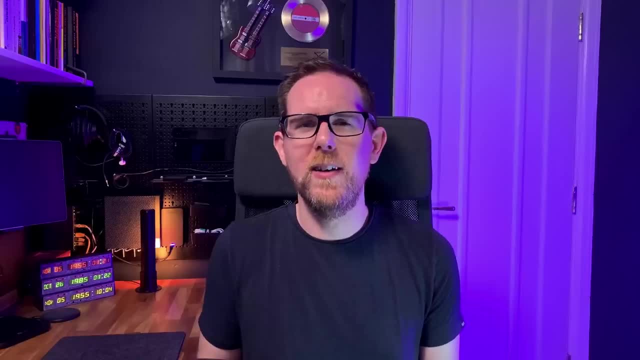 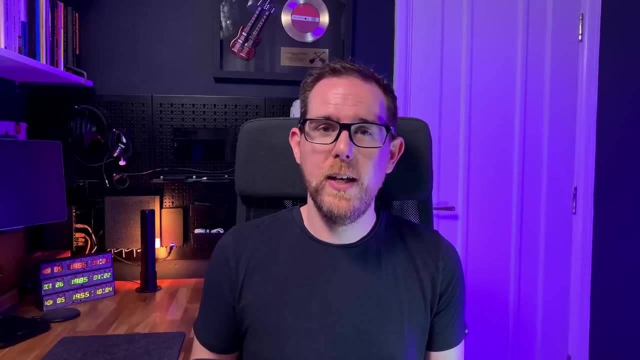 and being familiar with them, so that when you do have a problem you can think, oh, that sounds a bit similar to this design pattern, And then you can go look it up and learn a bit more and see if it applies. And the thing is out, of all of these different design patterns, there's only really 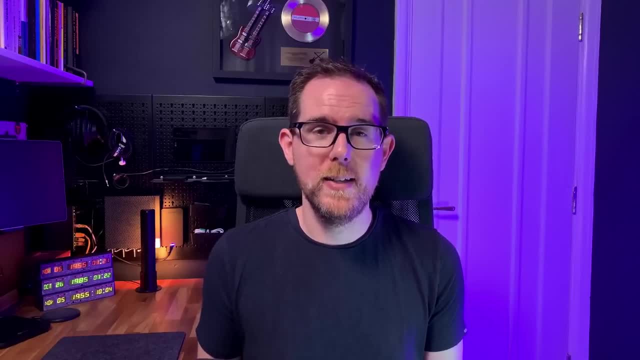 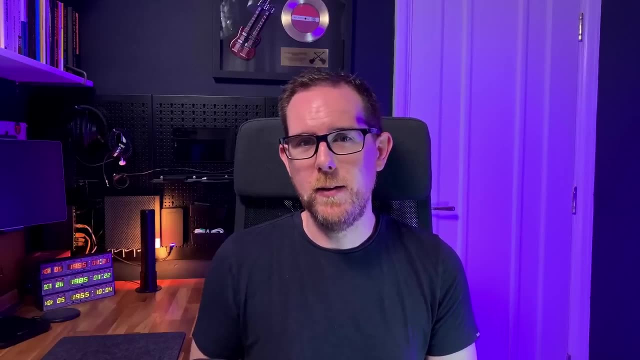 five that I find myself using over and over again. So let's have a look at those. So the first design pattern we're going to look at is the Creational Design Pattern. So the first design pattern we're going to look at is the Strategy Pattern. Now let's go back a bit to that cake baking analogy. 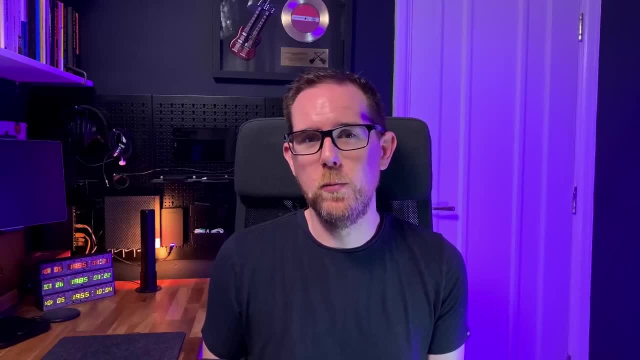 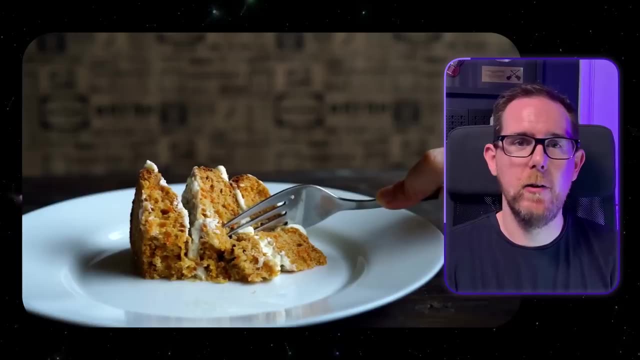 Let's say you love cake so much that you decide to write an application that will give you cake recipes. So let's say you start off with a birthday cake recipe but later you want to add in a red velvet cake and then a carrot cake. Now you could just do this with if statements and switch. 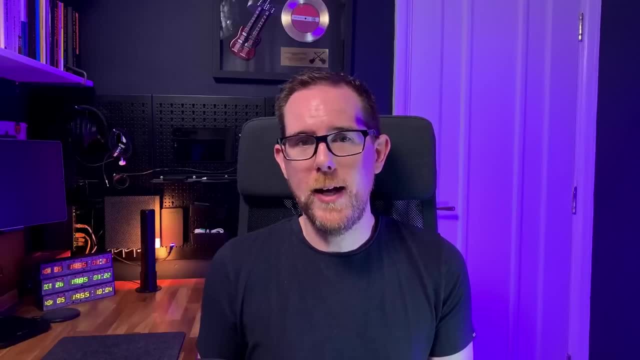 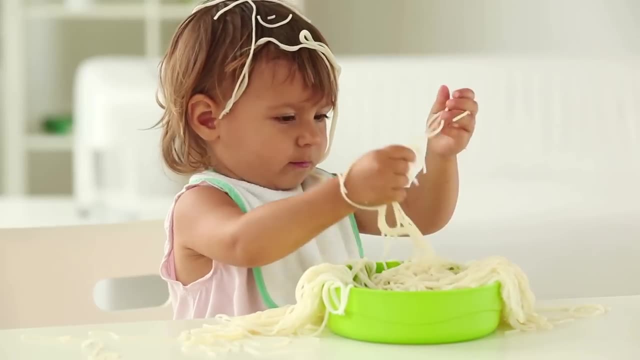 statements and add in all the cakes that way. But then you want to add in a coffee cake and a lemme cake and all of these different cakes and eventually your code ends up more like spaghetti than cake, going to get really, really messy. and the thing is the code in your application shouldn't really care. 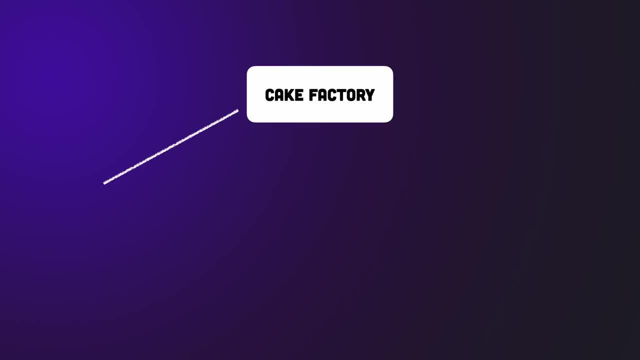 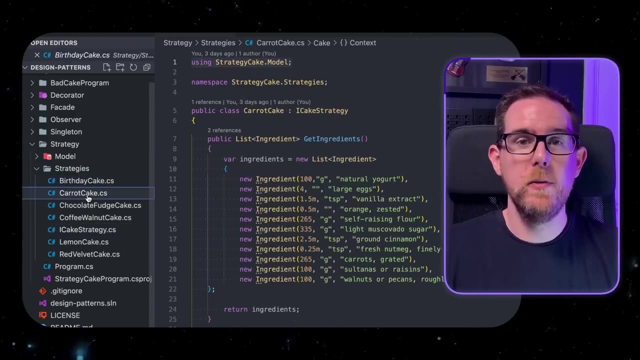 too much about which cake you pick. this is where the strategy pattern comes in. you can split all of those cakes into their own classes and have each of them implement the same methods, and then, when it comes to picking a cake, all you have to do is run two methods: get ingredients and. 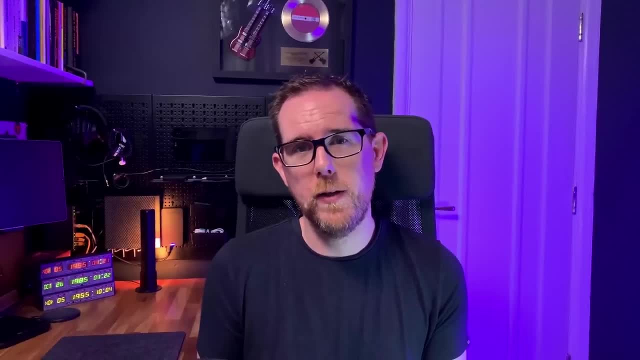 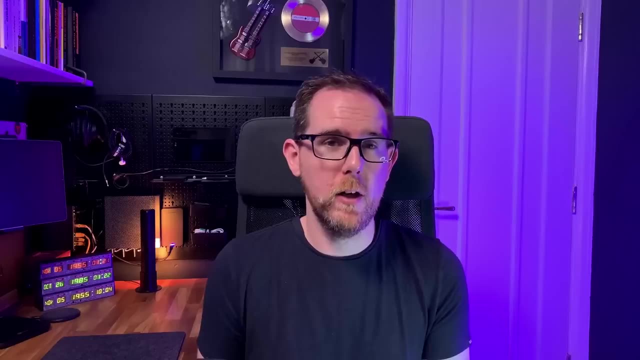 get method, and this is really useful if you have multiple ways of achieving the same thing in your application. let's say you've got a maps application and you want to provide navigation via walking, via car, via cycling. they're all going to have the same sort of functions, but the actual. 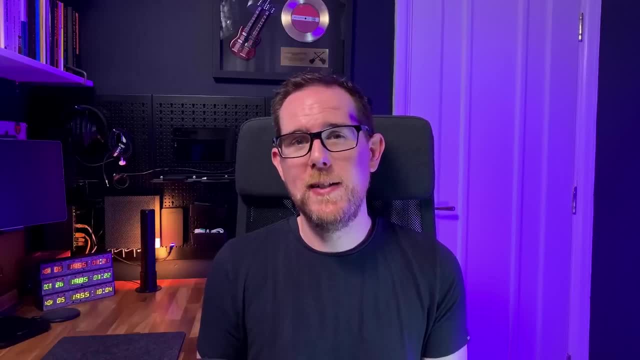 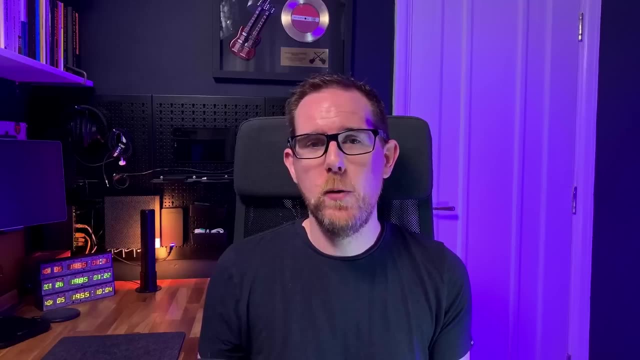 implementation is going to be different for each of them. this is definitely one pattern that's worth having in your toolbox to help you write clean code. the next pattern that i use the most is the decorator pattern. now, if you need to extend an object without actually changing the original, 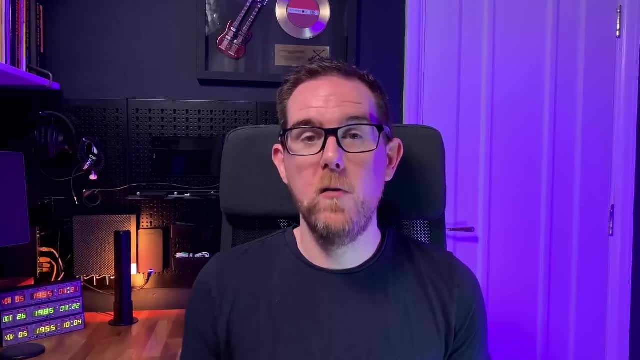 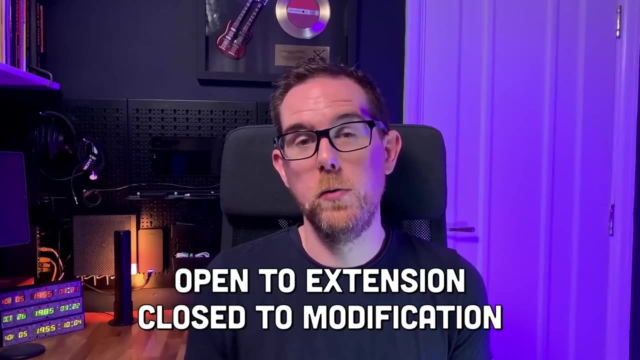 implementation, then the decorator pattern is one way to do that. now. i've mentioned the decorator pattern before in my video about solid, as it's one of the ways that you can make your code open to extension but close to modification. i'll put a link at the end of the video to the solid video if you haven't watched it already. 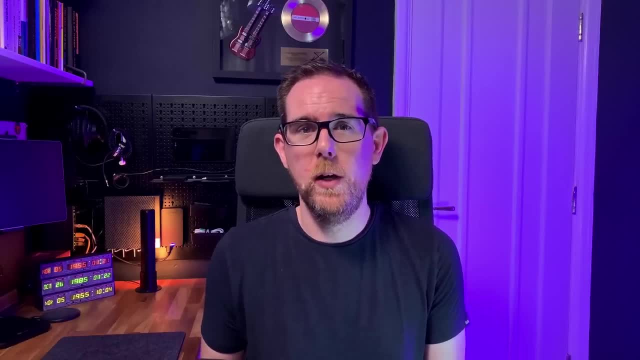 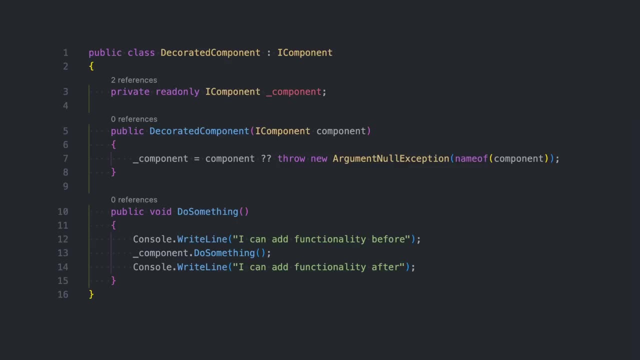 again, this is one of the patterns that i've used without realizing it before. whenever you wrap a class in another class, you're effectively using the decorator pattern. the way we normally do this is to have the decorator implement the same interface as the component you want to extend and then, in the decorator constructor, we take in that component. 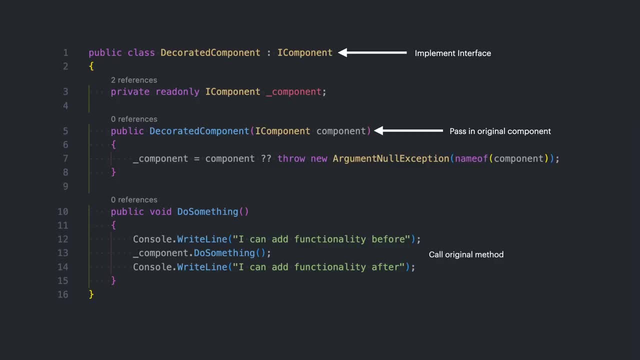 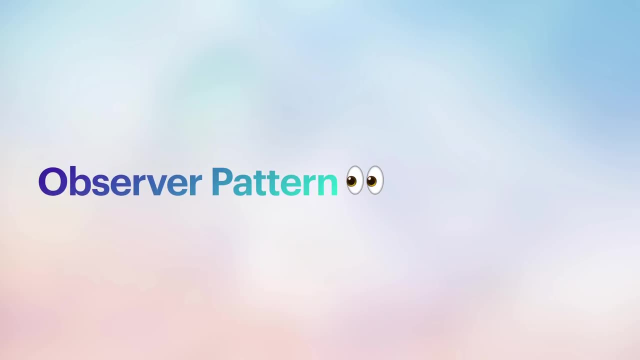 as an argument. you can then implement the interface and still be able to call the original component, but now you can add in additional functionality either before or after the you make that call. number three is the observer pattern. this pattern is something you're probably very familiar with already, even if you've never actually used this pattern before. the observer 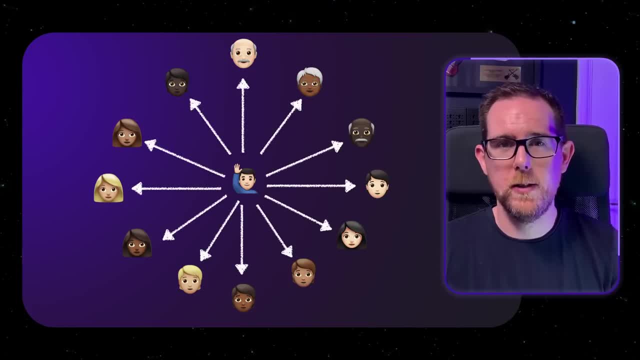 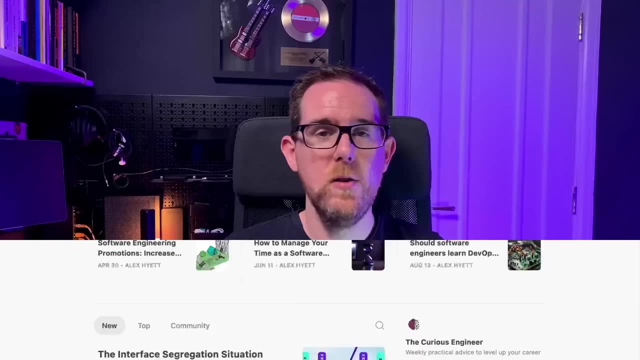 pattern is used whenever you want to notify interested parties that something has happened. if you're subscribed to my newsletter the curious engineer, then every sunday you will get an email from me. it's not sent to everyone who watches my youtube videos or reads my blog. it's only sent to 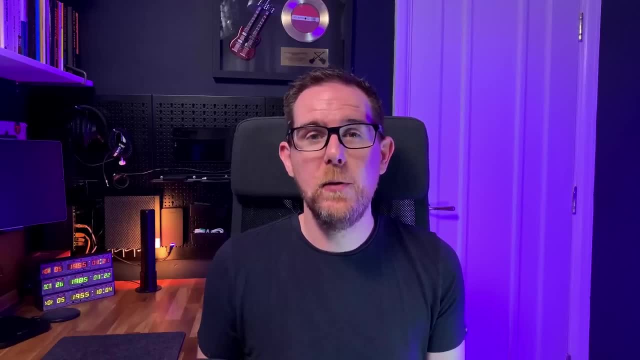 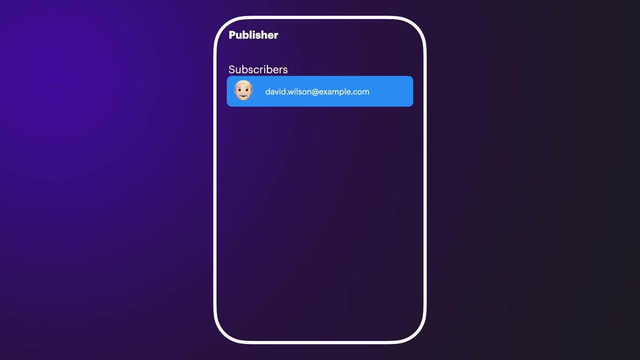 those select few who have subscribed to my newsletter. this is how the observer pattern works. so you have a subscriber- that's a publisher- that implements the subscribe, unsubscribe and notify subscriber methods. you then have a subscriber interface that all the subscribers need to implement to let the publisher notify them. when a subscriber subscribes to a publisher, they get. 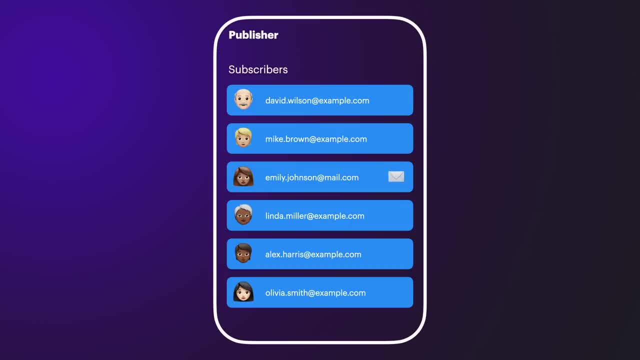 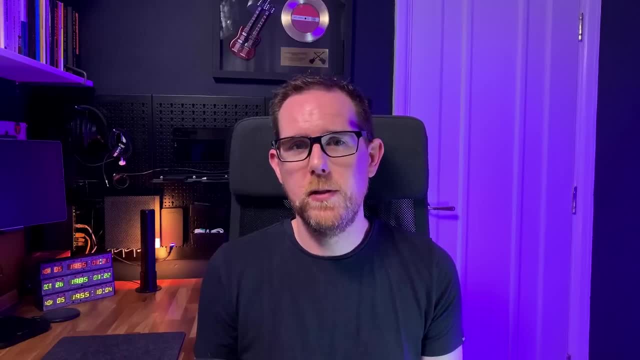 added to an array and then all the publisher needs to do is to loop through that array, calling the update method on all the subscribers. now our next pattern that we're going to look at is the singleton pattern. now, when we think about singletons, we think about creating one thing: 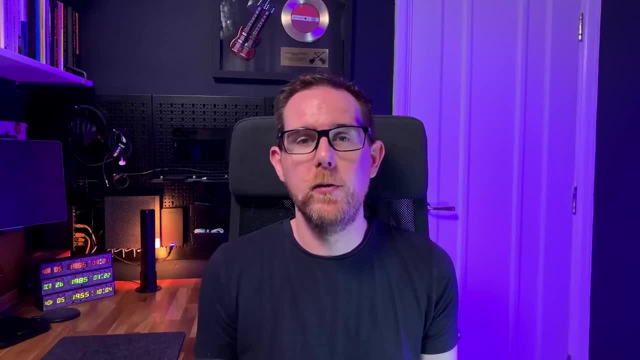 that's not a single object and that's a single object. the problem with that is that we don't have a single object everywhere, and that can be a problem with the data base you want to access. the problem with that is you can also change it anywhere, and that causes lots of different. 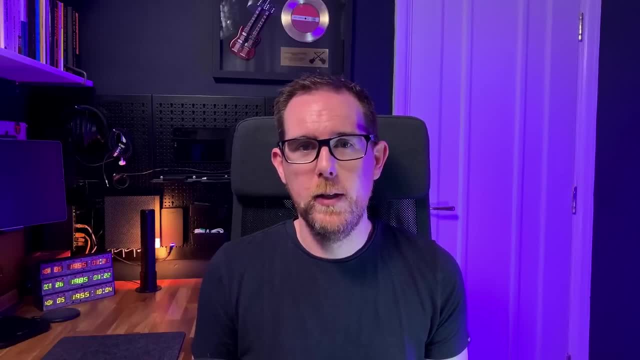 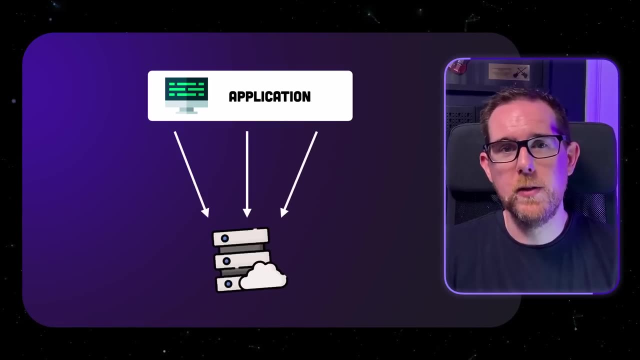 problems. but there are cases where we do need to have a single object and make sure that we have a single object everywhere, such as if you've got a database that you want to access. you don't want a different connection to the database for every single time that someone needs to use it. 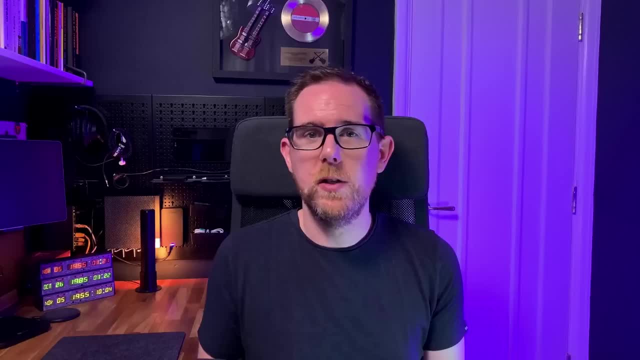 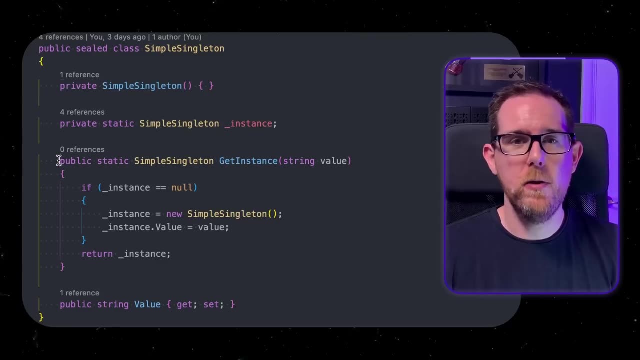 the typical way to do this is to create a sealed class with a private constructor can create a new instance of it, So you can't do new whatever. You then create a separate method or a property that lets you create an instance of that class. This is then stored in a static. 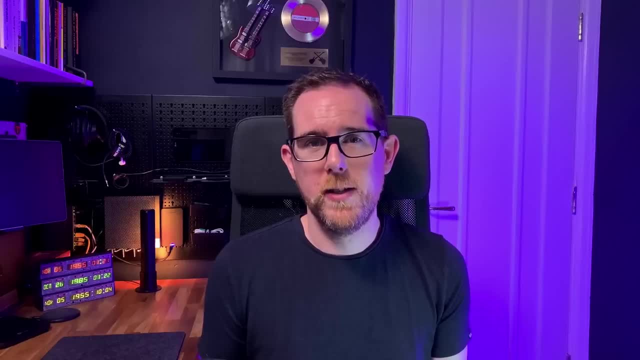 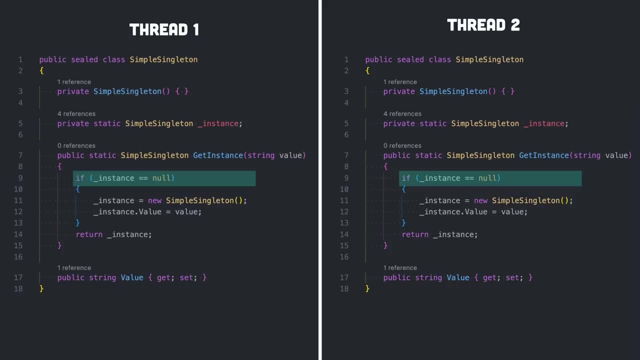 variable inside the class. The problem with this code is it's not thread safe. You can have two threads call this code at exactly the same time. They both reach that null check. The instance would be null and they'd end up creating two instances of the same object. Now to get around. 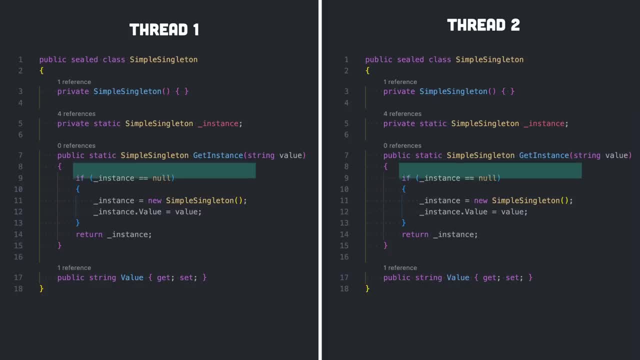 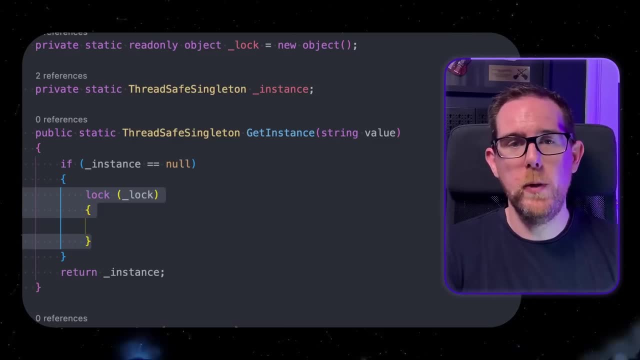 this. we need to have some form of locking mechanism. So we need a way to stop the other threads from accessing the code if one of the threads is already there. So to do this we have the same initial null check, but then we implement the lock and then we check again to see whether 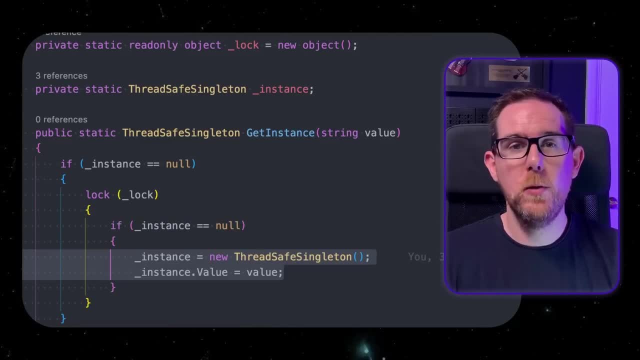 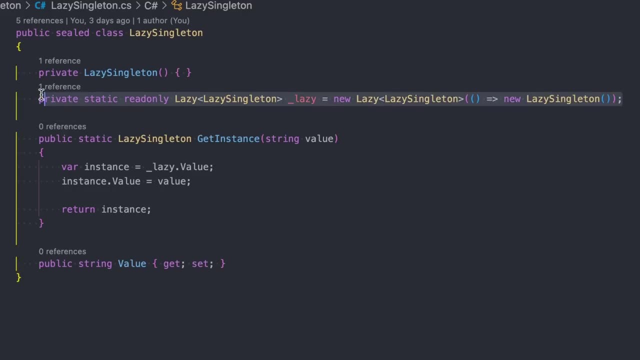 the instance is still null before then creating it, And this will prevent the two threads from creating separate instances of the object. Another way to do this, if you're using C sharp and NET 4, is with the lazy type. It's still thread safe, but it uses a lot less code. The last pattern that 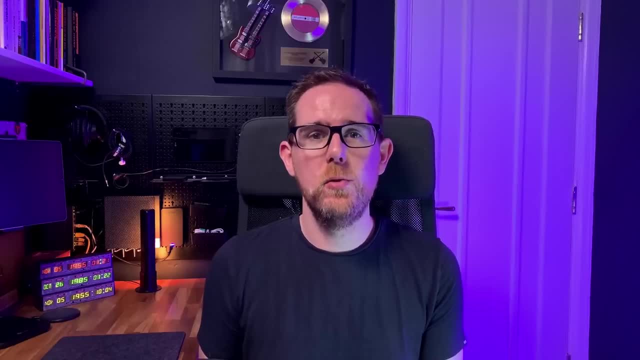 we're going to look at is the facade pattern. Now, this is one that's essential to software development and everyday life in general. The facade pattern is all about simplicity. We're constantly using different libraries and frameworks, and, even though they save us time, they can make our code messy and complicated. 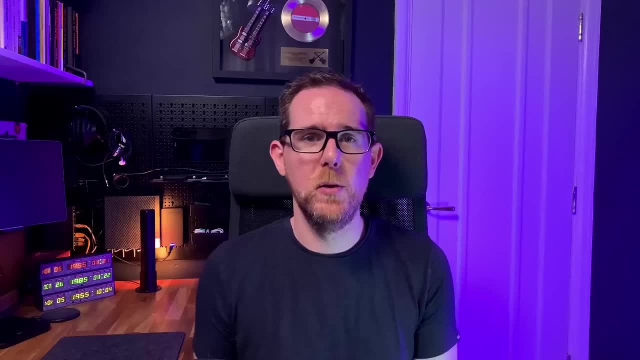 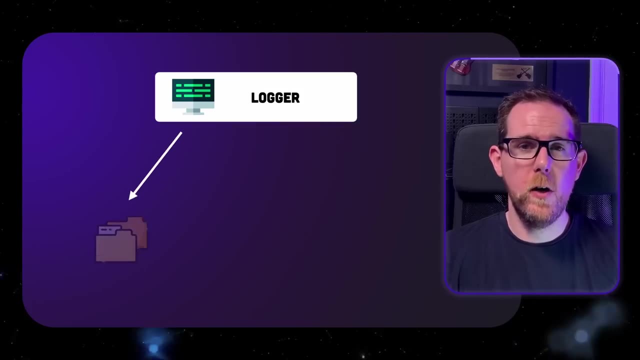 And in many cases the libraries do a lot more than we actually need them to do. Let's say you're making use of a fictional logging library that isn't very well designed. This library can send logs to a file, it can send it to the console and it can even send you a slack. 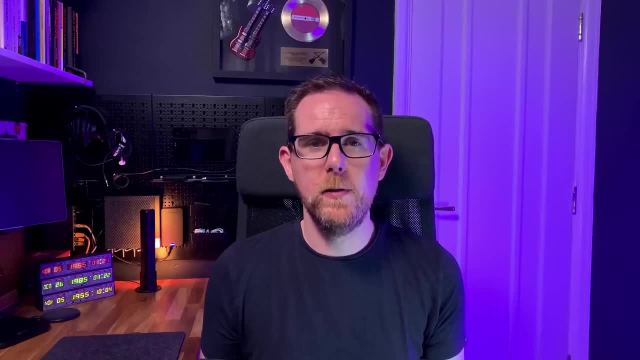 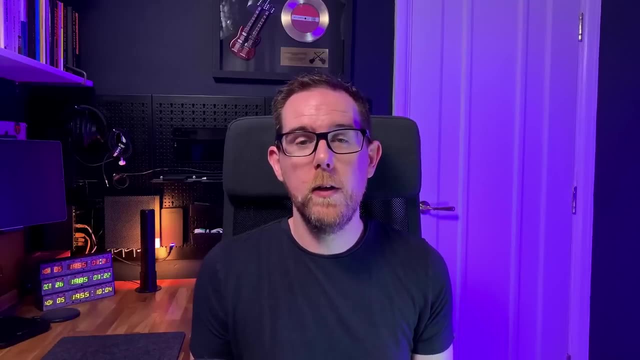 message. The problem is, this log library is not very well designed. It's not very well designed and it only has one method called log, And you have to specify with every single request what type of log message it is, as well as how you want to log it, Rather than clutter up your code with